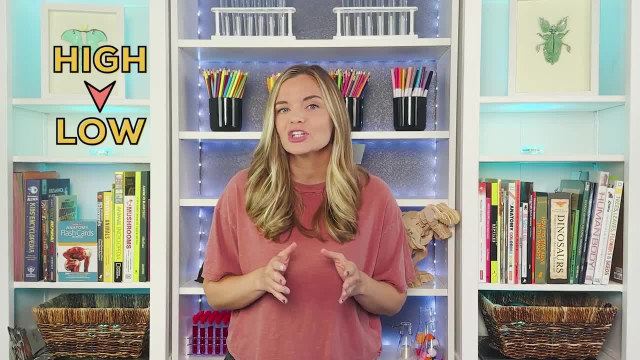 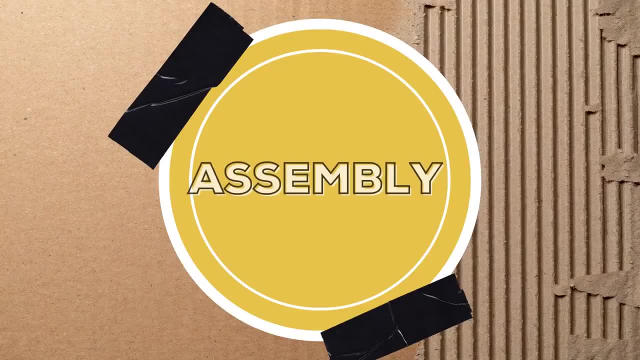 can also use a paper towel or a paper towel. You can also use a paper towel or a paper towel. You can wooden skewers. Energy moves from high pressure or temperature to low pressure or temperature, and the bigger the difference between the two, the faster it will move. 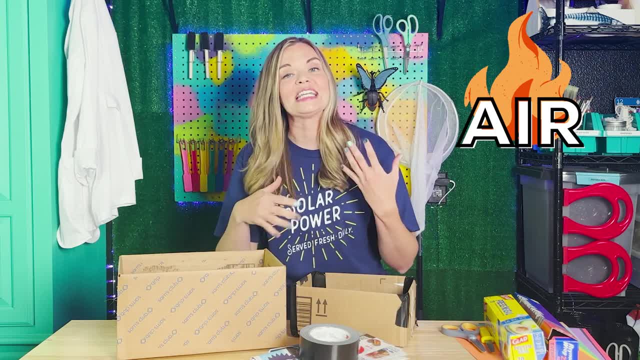 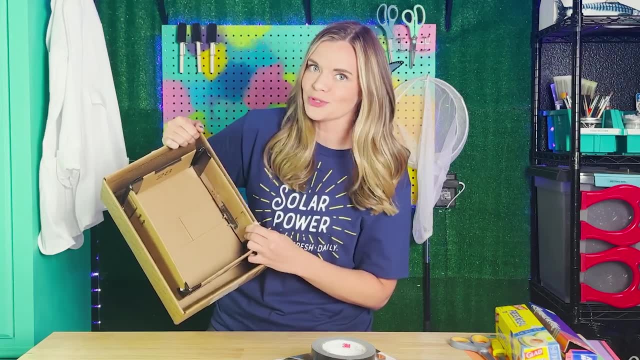 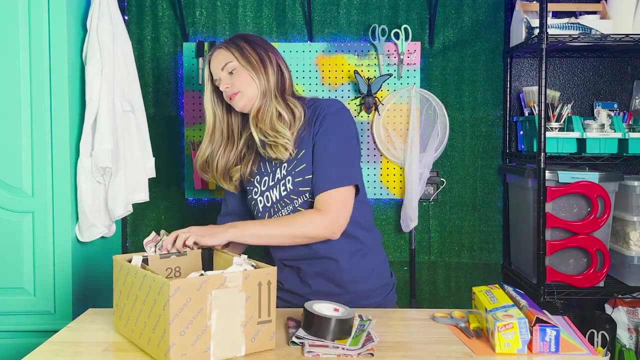 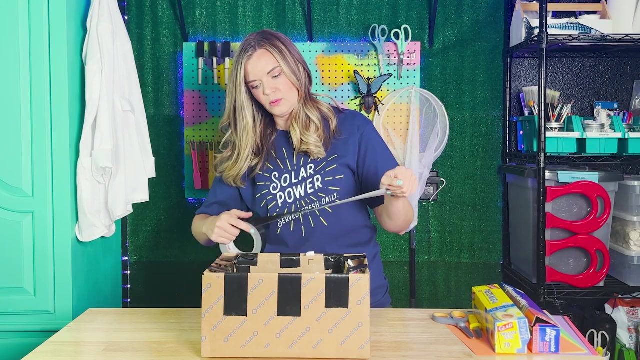 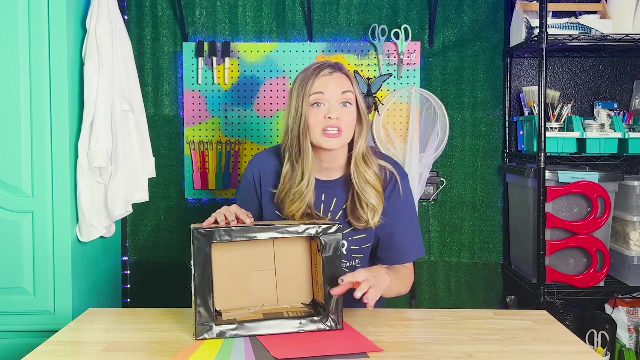 This means once the air inside of our oven begins to heat up, it will actively be trying to escape This space that we're creating between the two boxes. hopefully will slow that down. A We need to line the inside of our box with construction paper, but what color should? 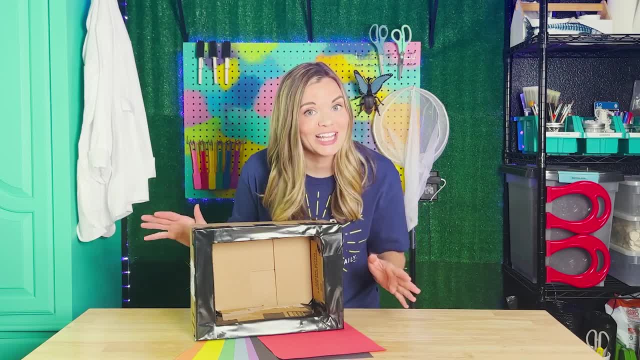 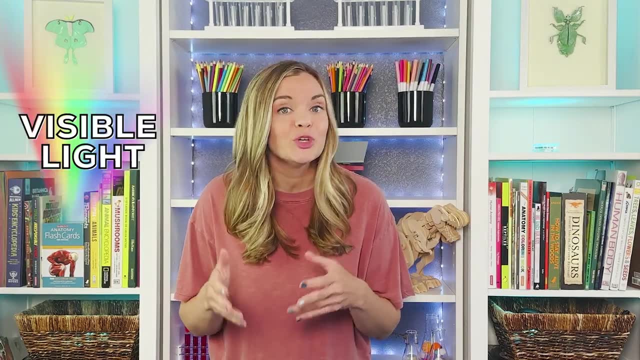 we use. We want our solar events to absorb as much light as possible. Light travels in waves. Some of those waves we can see and some we cannot. The visible light that humans see as the color white consists of a rainbow of colors. 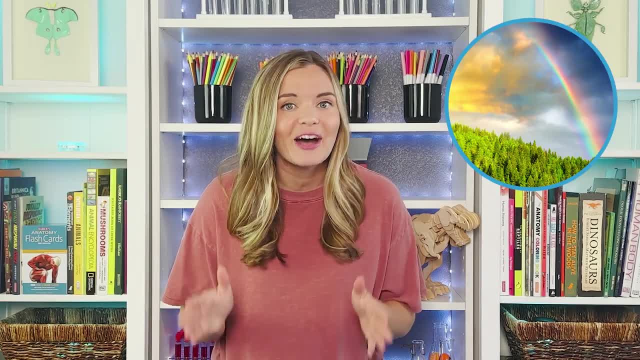 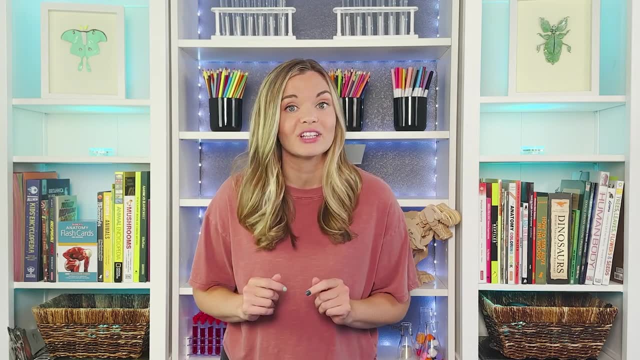 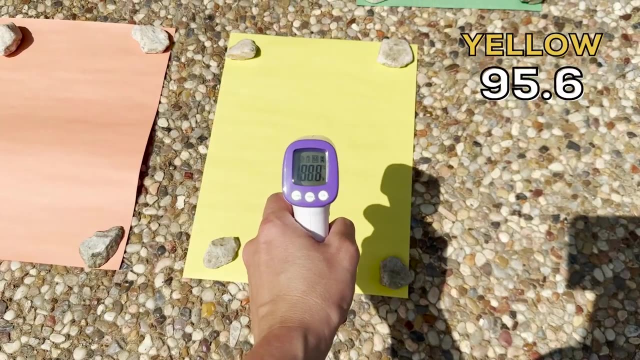 on the electromagnetic spectrum like a rainbow after a storm. If the color of a surface is anything other than white, it will absorb light from some of the wavelengths. I have an infrared thermometer that we will use to measure the temperature of each color. 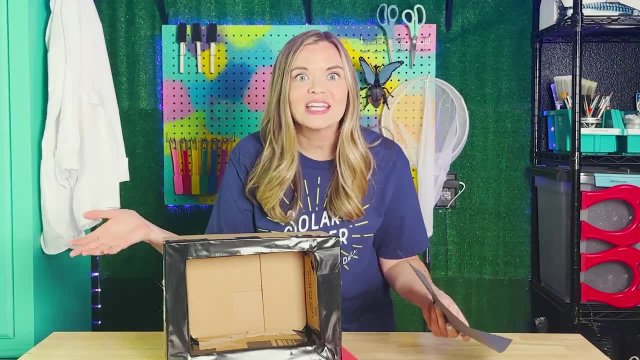 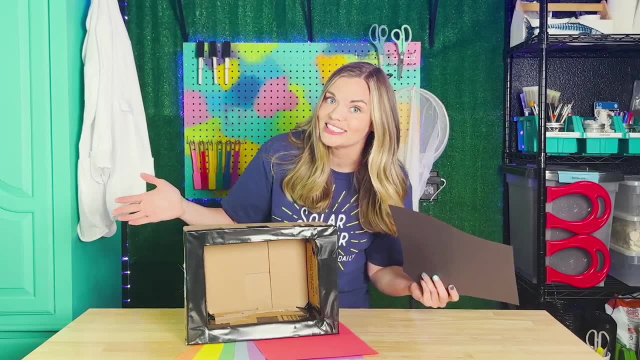 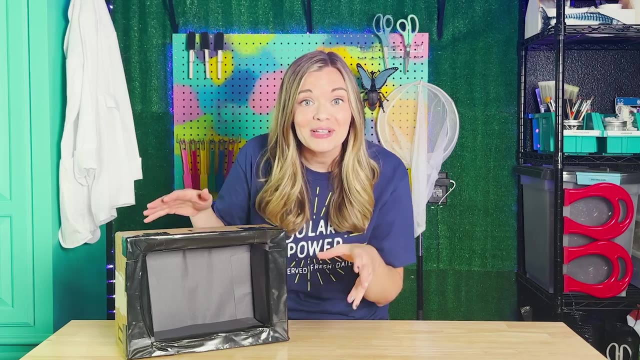 So black is the ultimate heat. This is because it absorbs all light on the visible spectrum, So this is what we need to use for our solar oven. Okay, now we need to figure out how to keep all of this energy inside of our box without 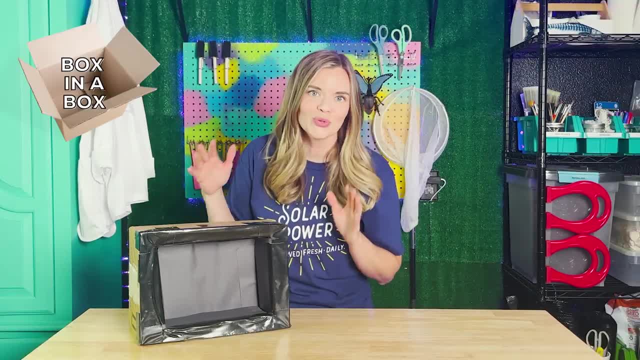 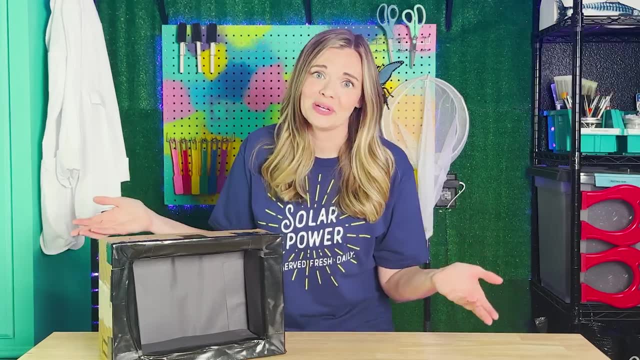 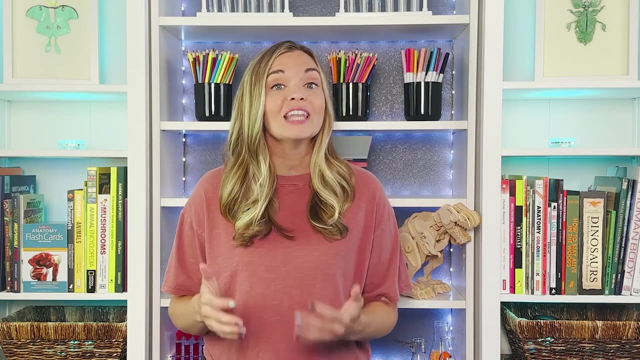 blocking the sun. Our box-in-a-box design is really going to help insulate the sides and the bottom, but light can't travel through those And that's why we need a solar oven, And that's a pretty big problem. Objects are either transparent, translucent or opaque, depending on the amount of light. 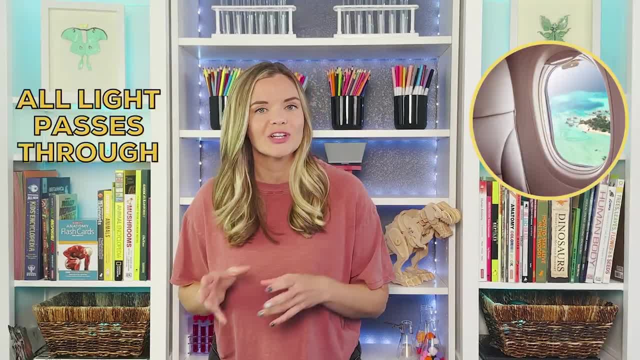 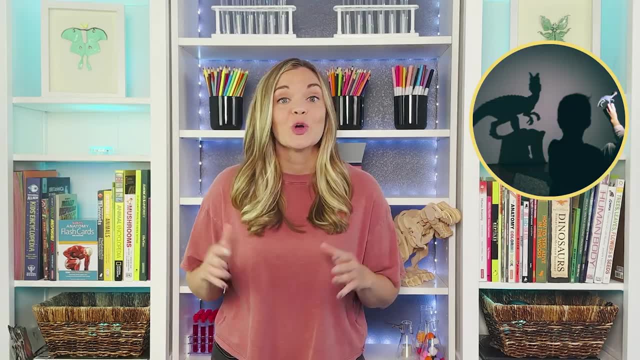 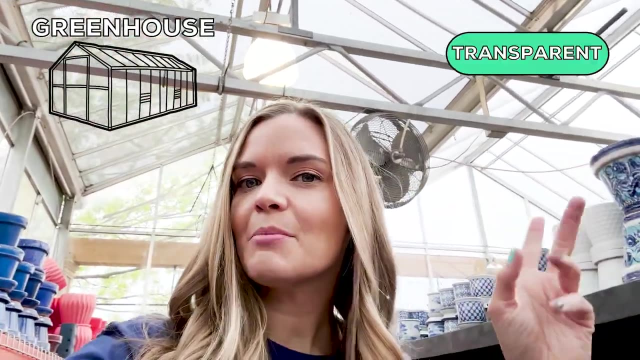 that is able to travel through them. Light travels through transparent objects, so you can see through them. Some objects are translucent, meaning they only let some light through, And opaque objects allow no light to pass through them. Some of the roof of this greenhouse is transparent and some of it is translucent, allowing the